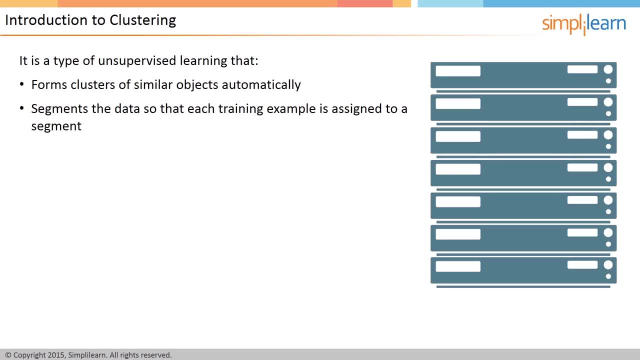 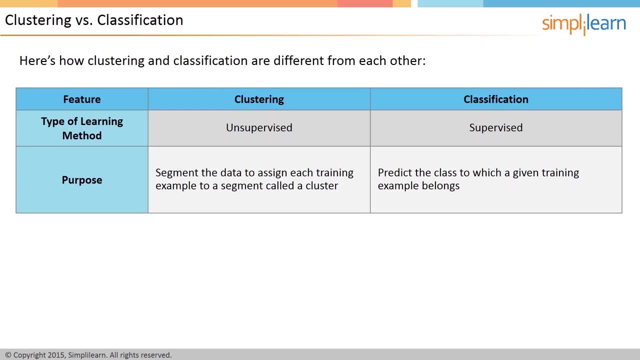 marketing, medical diagnostics and so on. This screen shows you the differences between classification and clustering. In classification, the training data has to specify what you are trying to determine, or the classification data has to specify what you are trying to determine. The training data can be used to certify what is in the menu By sure. 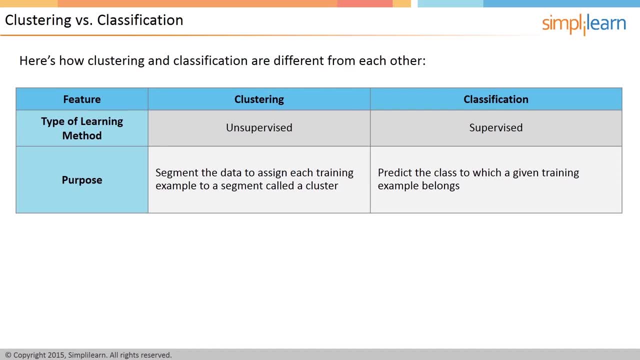 呼 is used in clustering. If a cluster is being brauchen Blood sorties at the end of a gave option, you can verify the tragings of the cluster shift in order to make sure the data runs well in the cluster. б- façon в которой data Mob knowledge get filtered. 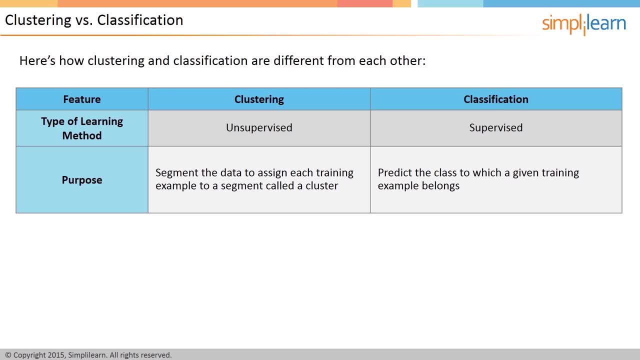 By Page. Angle 1, The chat naughty 2 caden on the test data. Examples are k-means and fuzzy clustering. The goal of classification is predictive, whereas the goal of clustering is descriptive. Distance measures and similarity measures are used to determine whether two objects 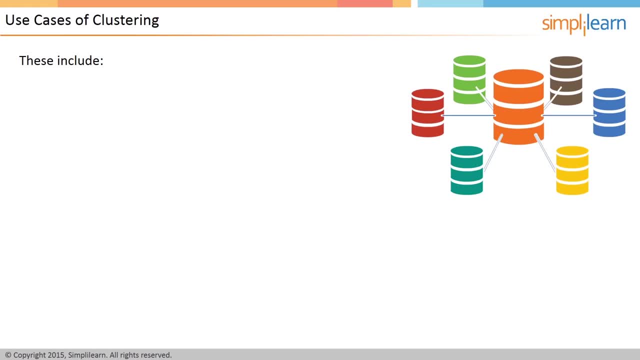 are similar or dissimilar. Now let's look at the use cases of clustering. Clustering models have many use cases that are the same as that for classification. A few of them are as follows: Grouping content on a website or products in a retail business. 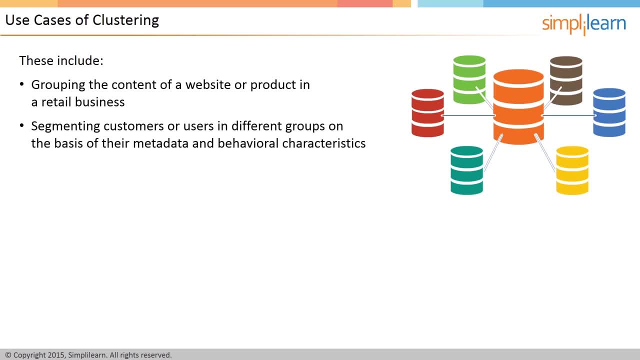 Segmenting users or customers into different groups based on behavior, characteristics and metadata. Segmenting communities in ecology. Finding clusters of similar genes. Creating image segments for use in image analysis applications such as object detection. The major clustering methods are distance-based, hierarchical partitioning and probabilistic. 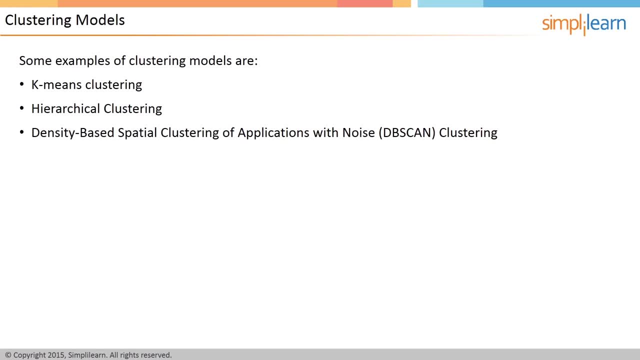 A good clustering model will give you clusters where the intraclass similarity is high and the interclass similarity is low. In distance-based method for continuous valued variables, the distance between two instances can be measured by estimating the Minkowski metric or the Euclidean distance you saw earlier. 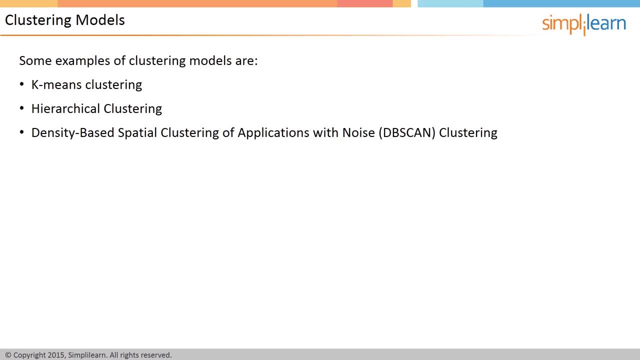 in the course. Standardizing data can help mitigate the effects of the choice of measurement unit on the clustering analysis. You can use contingency tables for binary attributes, Simple matching for nominal attributes, mapping the range of ordinal attributes onto 0,, 1,. 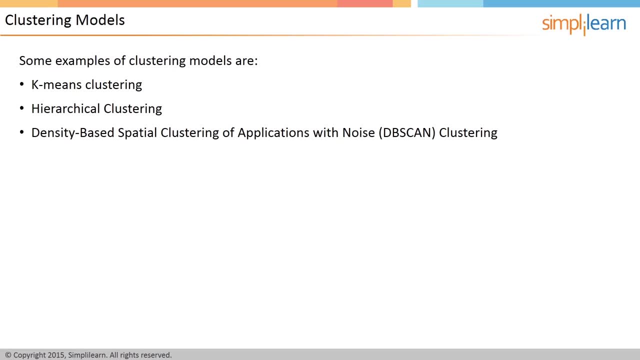 and treating them as numeric and combining the methods for mixed-type attributes. An alternative concept is the similarity function, which compares two vectors. There are various similarity measures, such as the cosine measure, Pearson correlation measure, Jaccard measure and Dice coefficient measure. 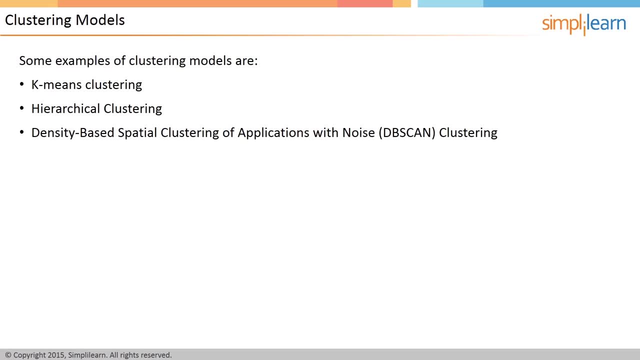 Several evaluation criteria, both internal and external, exist to decide whether the data is good clustering or not. Internal quality criteria judge the intracluster homogeneity and or the intercluster separability using any of the following: Sum of squared error or SSE minimum variance criteria. criteria Condorcet's criterion. 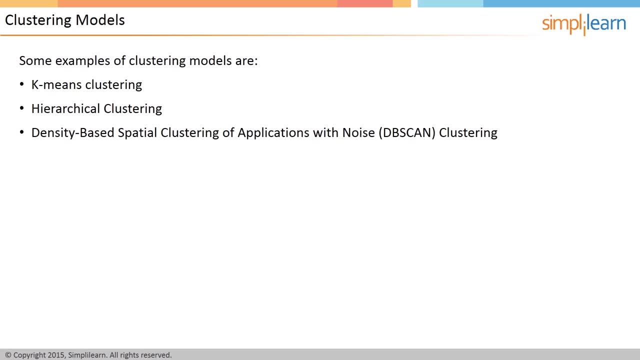 category, utility metric and edge cut metric. What an external quality criterion does is that it works out whether cluster structure matches some pre-specified classification of instances used in the analysis. For example, if the cluster structure matches some pre-specified classification of instances. 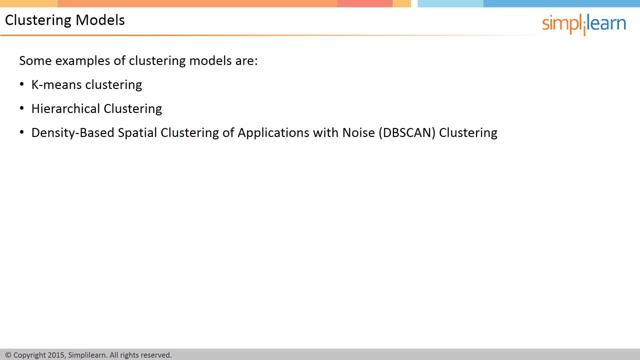 used in the analysis. it can be used to determine whether the cluster structure matches some pre-specified classification of instances used in the analysis. In the subsequent screens you can get an overview about the clustering methods. Many clustering methods are in existence, each using a singular induction principle. 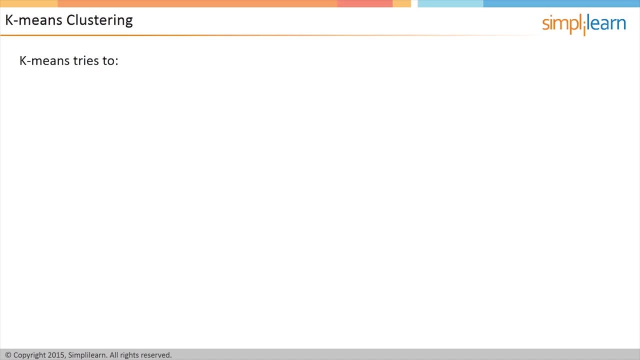 Farley and Rafferty divides them into hierarchical and partitioning methods. Han and Camber suggested three additional groups: density-based methods or DB scan, model-based clustering and grid-based methods. Estiville-Castro suggests classification based on the various induction principles used. 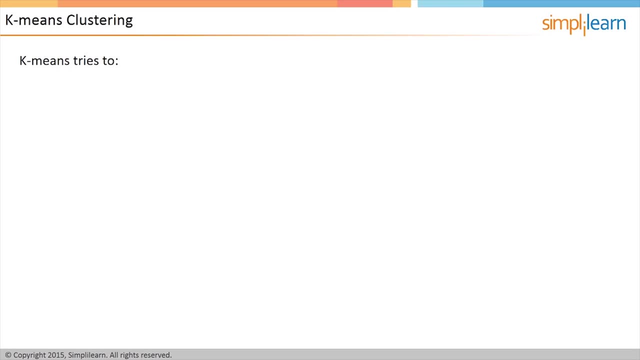 There are various classifications for the clustering algorithms as well. K-means clustering, an exclusive clustering algorithm, that is, data is grouped in such a manner that one object belongs only to one specific cluster. Conceptually, this is perhaps the simplest method that can be used on new data. 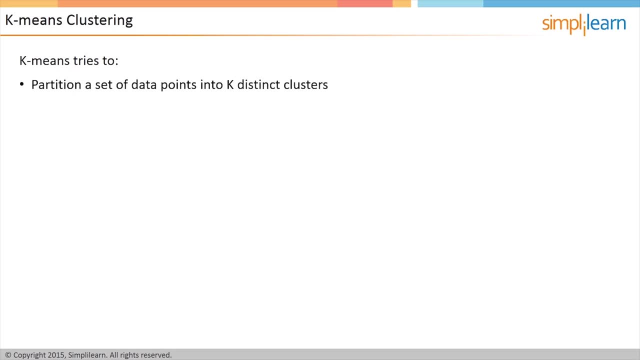 However, it is not suitable for nominal data. K-means is a partitioning method. Here, n objects are partitioned into k clusters such that each datum belongs to the cluster with the nearest mean. There will be the greatest possible distinction for k different clusters. 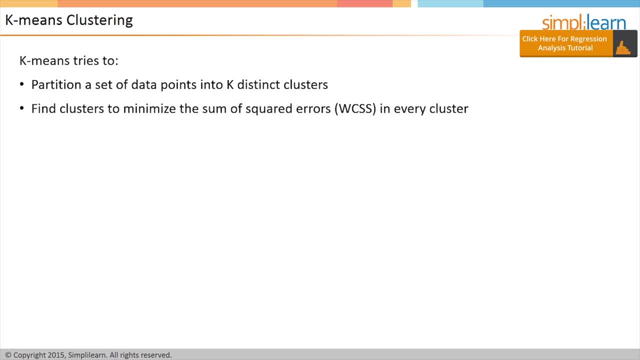 K-means tries to find clusters to minimize the sum of squared errors in every cluster. This objective function is known as the within-cluster sum of squared errors, or WCSS. The formula for computing WCSS is shown on the screen. However, the k-means method is sensitive to outliers. 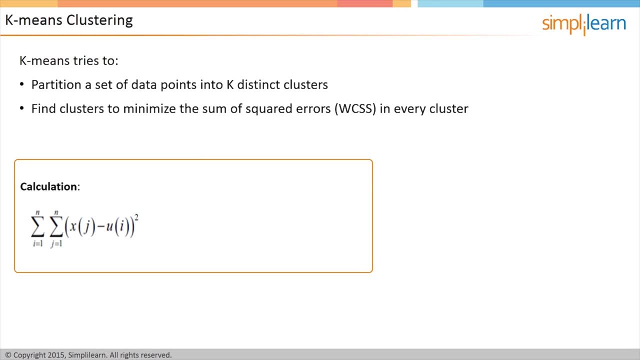 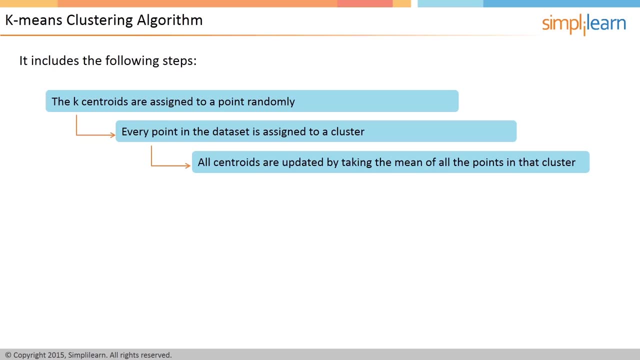 You can use k-metoids instead. This is a hard algorithm, which means that one instance is assigned to only one cluster. It is a flat algorithm, that is, all clusters are the same. This algorithm is iterative, wherein the initial cluster set is improved by reassigning instances. 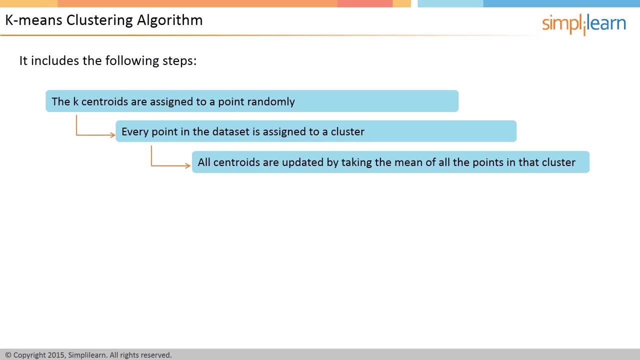 This algorithm partitions the data into k clusters represented by the initial cluster set. Each cluster center is calculated as the mean of all instances which belong to that cluster. You need to decide the number of clusters in advance, which could be a problem as there is no global theoretical way to identify the optimal number of clusters. 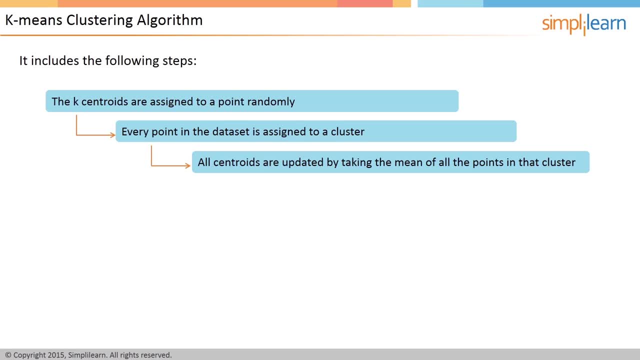 Consider an example: There are 16,000 rows of data in the data set and we need 4 clusters. Then we will create the first- k equals 4- initial cluster by selecting 4 records randomly from the data set. Each of the 4 initial clusters will have only one row of data. 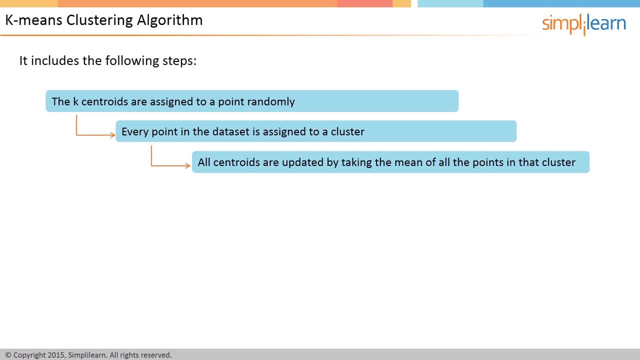 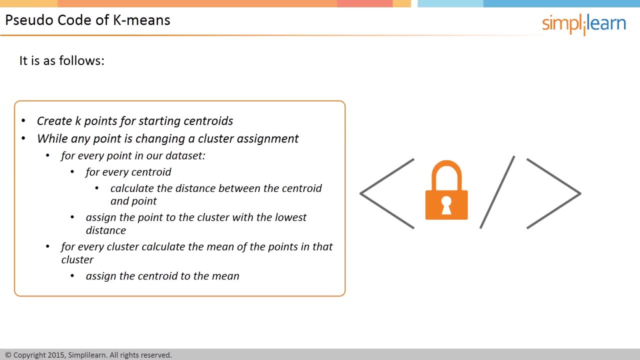 The intuitive formulation of the k-algorithm is shown on the screen. Set the number of clusters you want to generate, that is k. Choose k points randomly as the centers of these clusters, Using Euclidean distance or a similarity measure. assign each record to its nearest cluster. 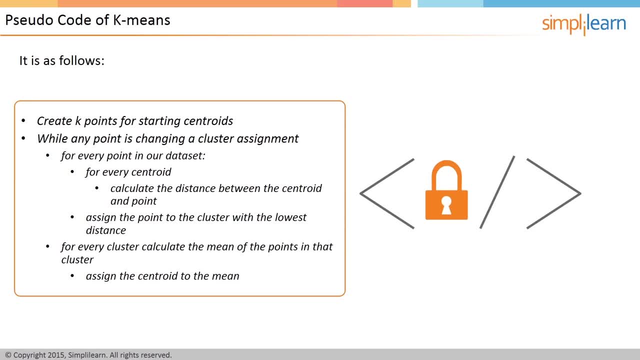 Calculate the mean, that is, the centroid, for every cluster and its nearest cluster. This is a very simple method. Let's try it. Set k for every cluster and use it as the new cluster center. Then reassign the instances to the closest cluster center. 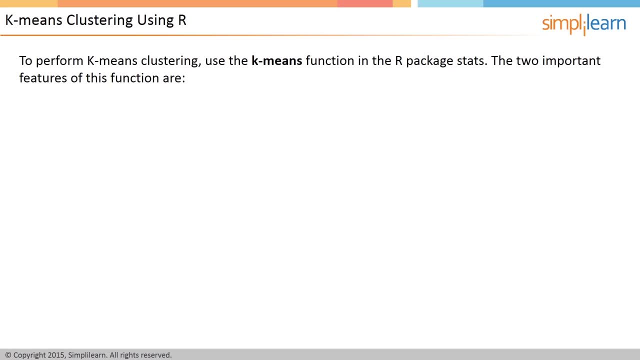 Iterate until there is no change in the cluster centers. Let's now see how we do k-means clustering using R. R has an array of options for clustering. We can use the function for k-means in the R package stats. This algorithm is known to be fast and reliable. 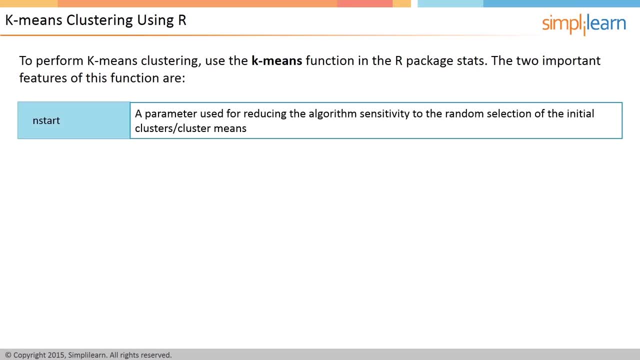 The parameter nstart can be used to reduce the sensitivity of the algorithm to the random selection of the initial cluster's cluster means. If the argument centers is number, then nstart will decide how many random sets should be chosen. Also, note that the cluster labels 1,, 2, and so on usually change from one run to the other. 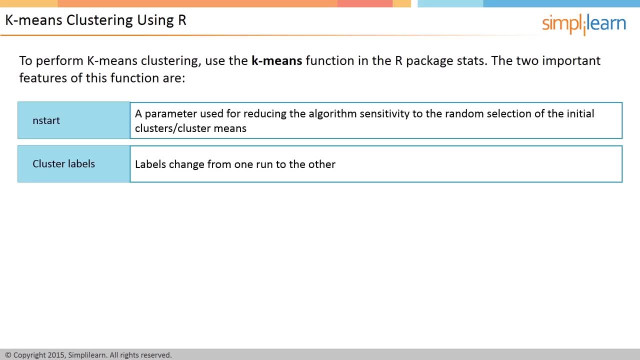 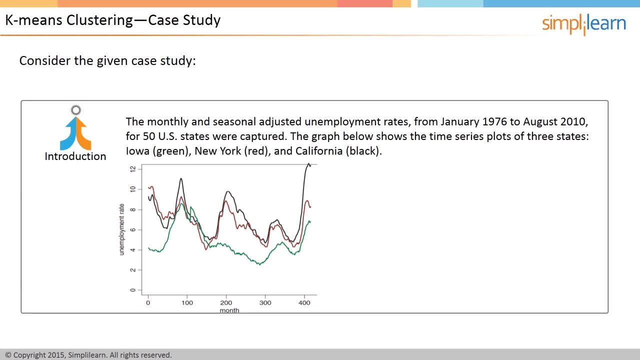 This only has to do with the labeling of the clusters, but not with the assignment of the elements to the clusters. Let's see a case study to see how we can apply k-means. We can analyze monthly seasonal adjusted unemployment rates covering the period January 1976 through August 2010 for the 50 US states. n equals 50.. 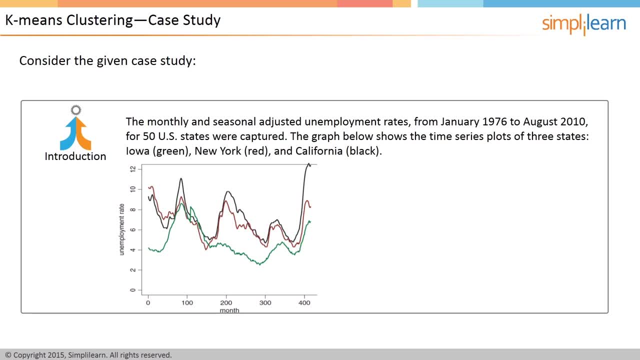 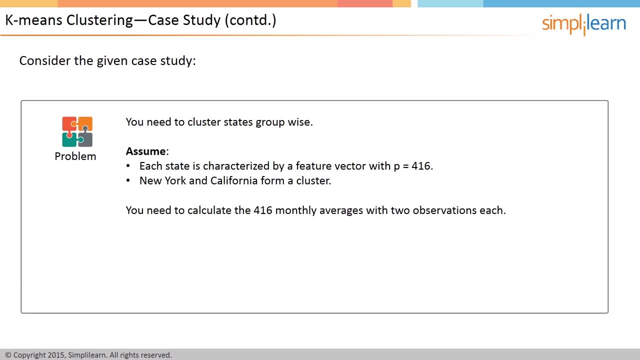 In the figure shown below we overlay the time series plots of three states: Iowa green, New York red and California black. The objective is to cluster states into groups that are alike. Here each state is characterized by a feature vector of very large dimension. 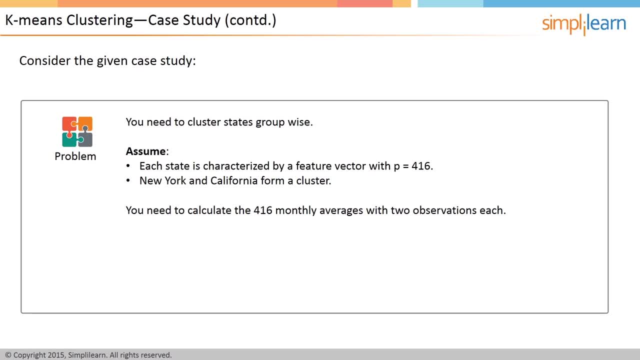 or p equals 416,, with its components representing the 416 monthly observations. Assume, for illustration, that New York and California form a cluster. You need to calculate the 416 monthly averages of two observations each. This vector of averages is the centroid for that cluster. 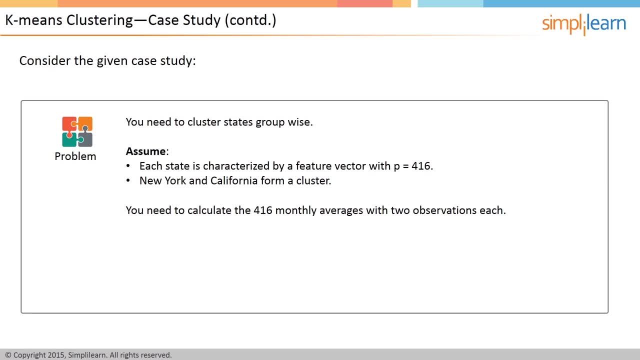 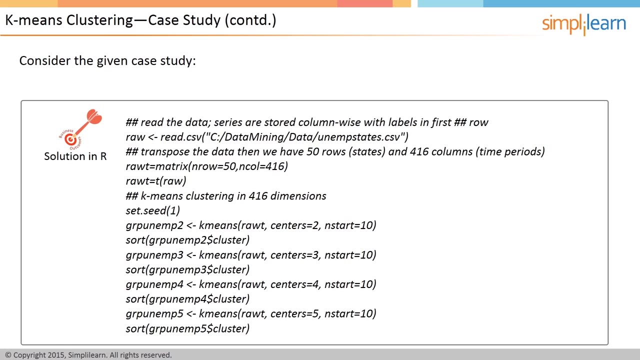 The sum of the squared distances from the centroid of this cluster- for New York and California there are 2- into 416, equals 832 such distances, which expresses the within-cluster sum of squares. Let's see how to perform k-means clustering in R. 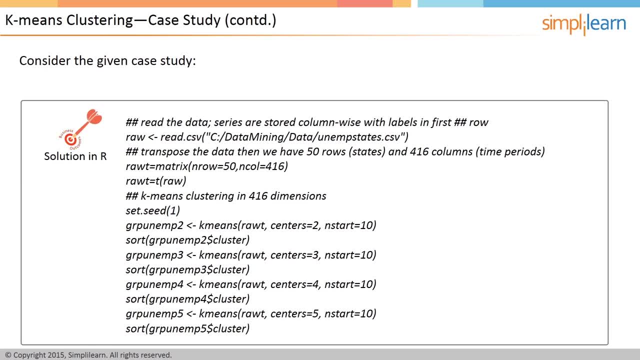 1. You need to use readcsv in order to read the data. 2. Transpose the data as matrix of 50 rows or states and 416 columns or time periods. 3. Then create k-means cluster with 416 dimensions by using the k-means function. 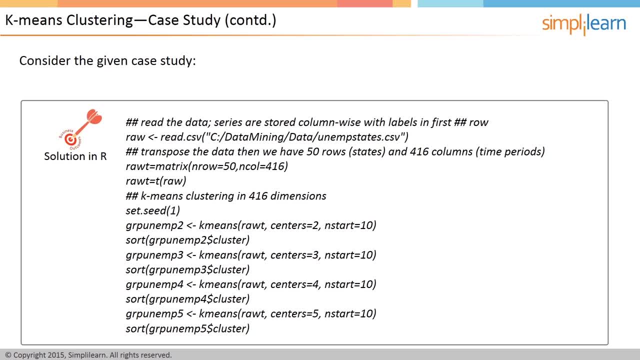 The format of the k-means function in R is k-means x centers, where x is a numeric data set matrix or data frame, and configurations and reports on the best one. For example, adding nstart equals 10 will generate 10 initial configurations. 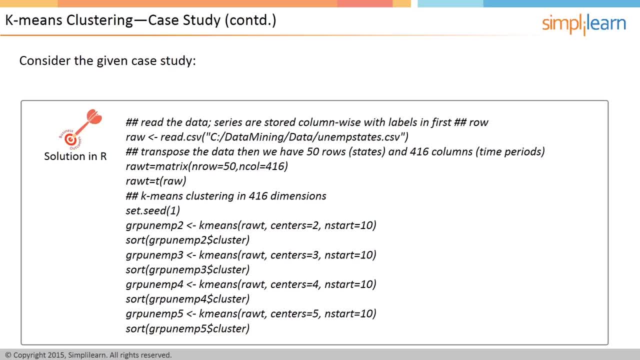 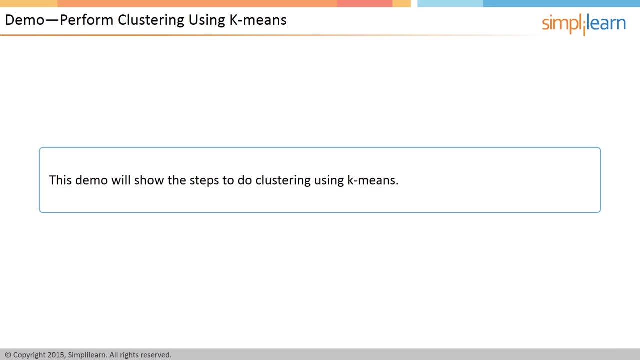 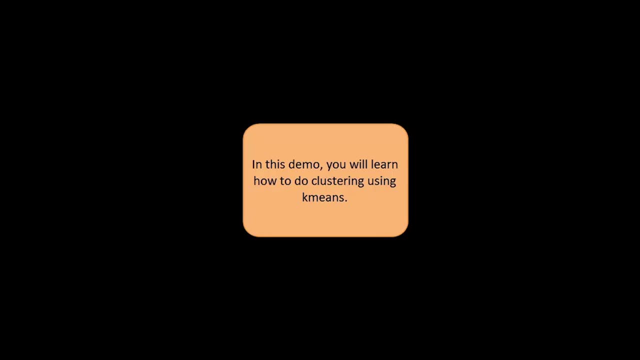 This approach is often recommended 4.. Similarly, you should create 2,, 3,, 4, and 5 clusters with nstart equals 10.. This demo will show the steps to do clustering using k-means. In this demo, you'll learn how to do clustering using k-means. 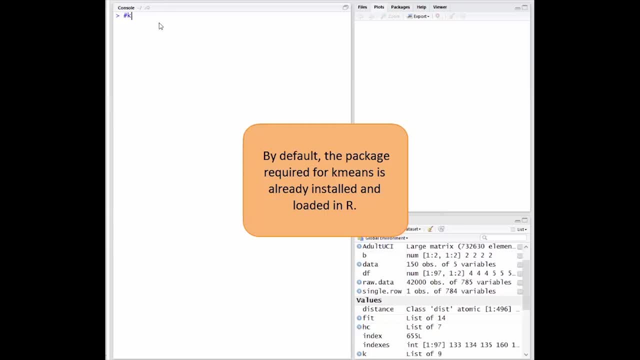 By default, the package required for k-means is already installed and loaded in R. For this demo, we'll use the data set called iris, which is already loaded in R by default. Let's prepare the data set by removing unnecessary column species from the iris data. 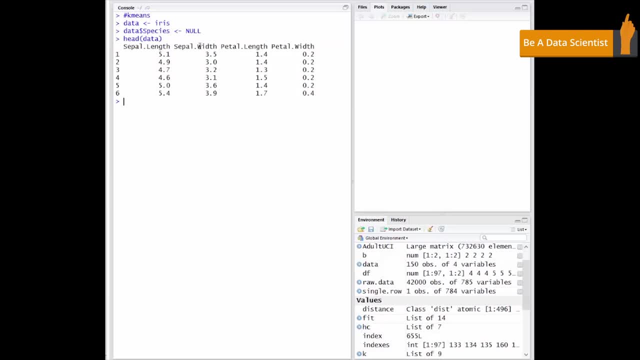 We can use the k-means function to do the clustering in that data. Here are some examples of the function in R. If we want to add a new column species to our data set, we'll use the array to be added in our data set. 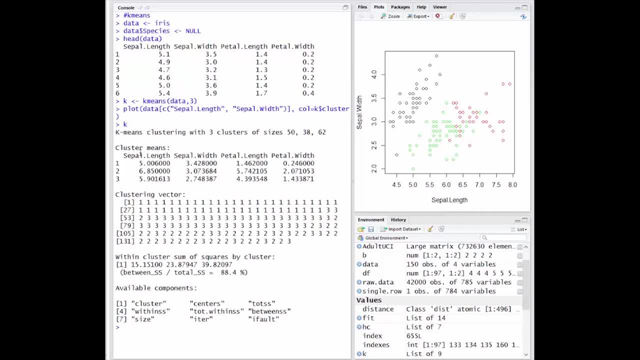 By default, the data set we'll be reminder of is not used in the program, but we can add it to the pretest in the data set over here. For example, we can add an array to the data set in the program which will be added in the program. 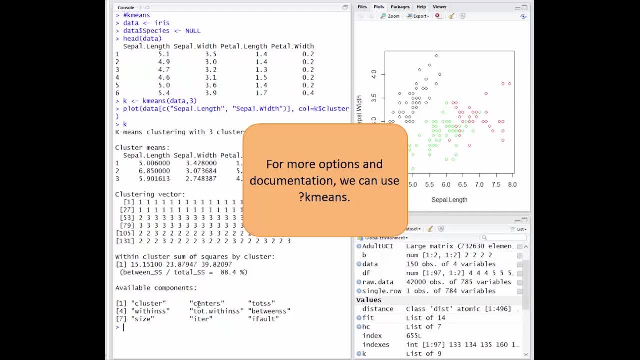 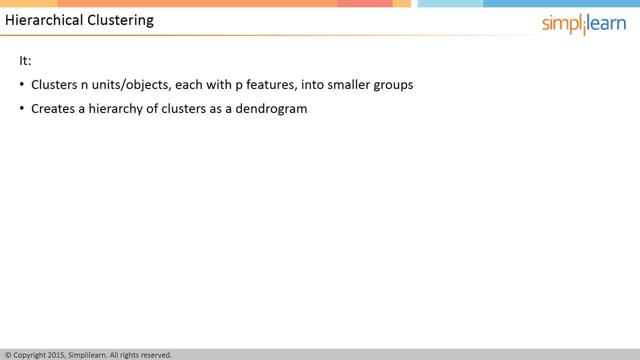 For more options and documentation, we can use the given function In this screen. we'll look at hierarchical clustering. In this method, you recursively partition the instances. This is done in either a bottom-up or top-down fashion to give you a dendrogram as a result. 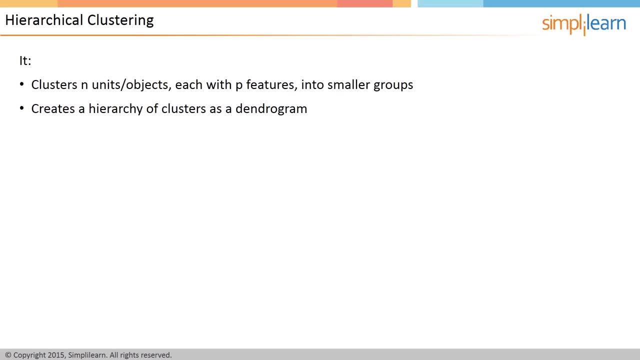 From a single cluster containing all objects to n clusters that each contain a single object is what partitioning in several steps gives you. Dendrograms are quite useful as they give us a visual representation of the clusters In the dendrogram. units in the same cluster are joined by a horizontal line with the. 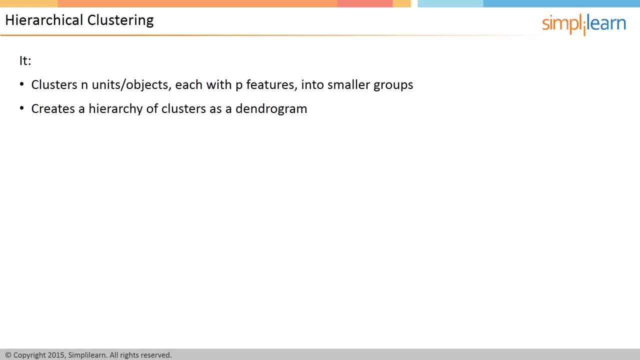 scale on the y-axis of the dendrogram reflecting a measure of the distances of the units within the cluster. The leaves at the bottom of the dendrogram represent the individual units. Leaves are combined to form small branches. Small branches are combined into larger branches until one reaches the trunk or root of the. 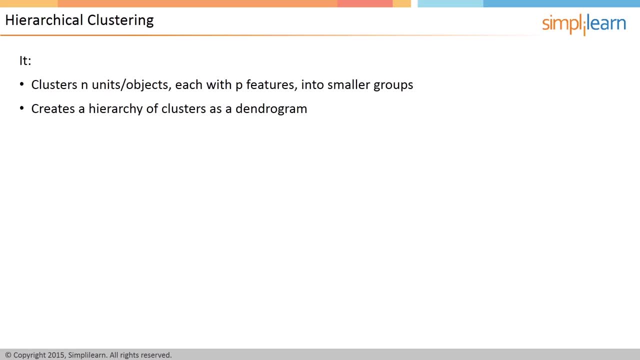 tree. that represents a single tree. The leaves at the bottom of the dendrogram represent the individual units. Important points about dendrograms. Units in the same cluster are joined by a horizontal line. The leaves at the bottom represent individual units. They are useful as they provide a visual representation of clusters. 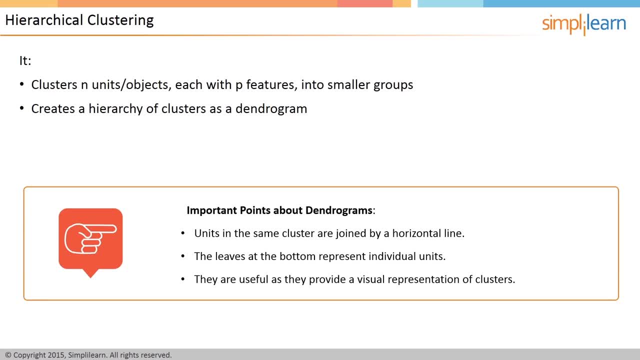 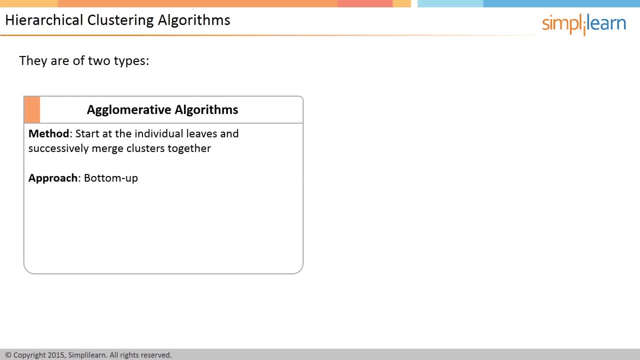 Next we'll look at the two major hierarchical clustering algorithms. Algorithms for hierarchical clustering are either agglomerative, in which we start at the individual leaves and successfully merge the clusters together, Or divisive, in which we start at the root and recursively split the clusters. 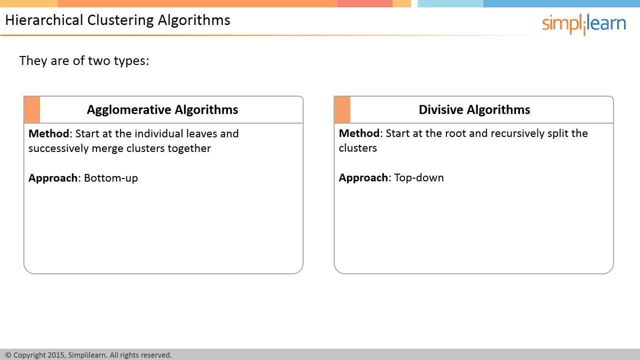 Agglomerative clustering is a bottom-up approach. In this method, initially each item is in its own cluster and then iteratively clusters are merged together. Divisive clustering is a top-down approach. In this method, initially all items are in one cluster and large clusters are successfully. 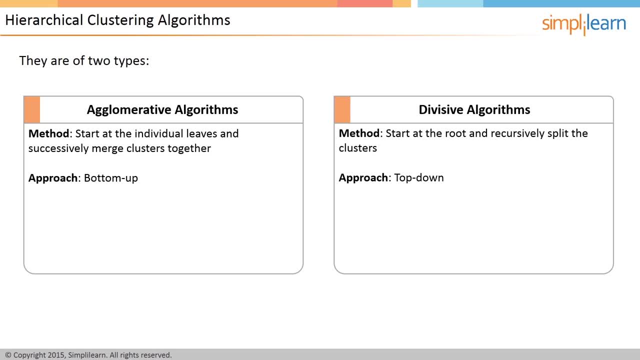 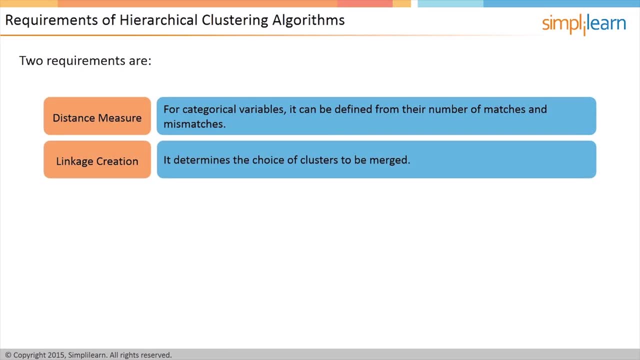 divided. Both methods produce a dendrogram. Hierarchical clustering procedures. Clustering procedures require both a distance measure and a linkage criterion. The tree clustering method uses the similarities or distances between objects when forming the clusters. Euclidean distance or squared Euclidean distance gives you the geometric distance in multidimensional. 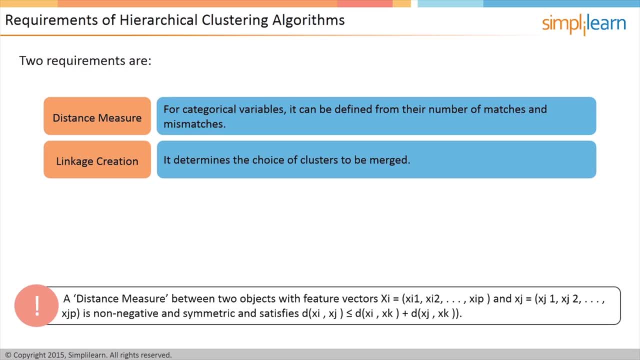 space. Other measures are the city block distance, Chebyshev distance and power distance. Percent disagreement can be used for categorical data. Once the distance measure tells you the distances between objects in a cluster, you can start with heading a levers based order. 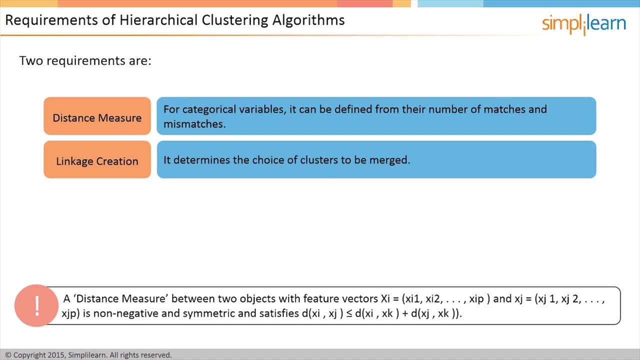 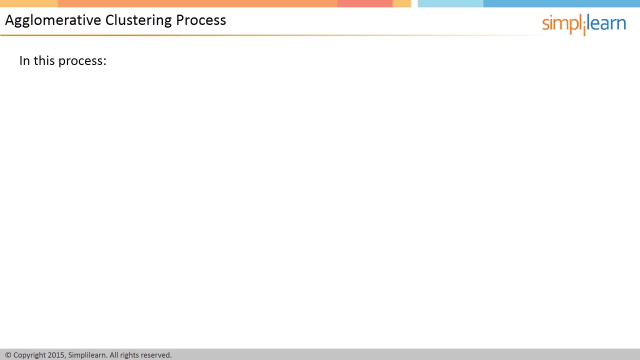 In this: 2. to any member of the other cluster. In average linkage clustering, the distance between one cluster and another cluster is equal to the average distance from any member of one cluster to any member of the other cluster. You can see how agglomerative clustering is implemented in computers. 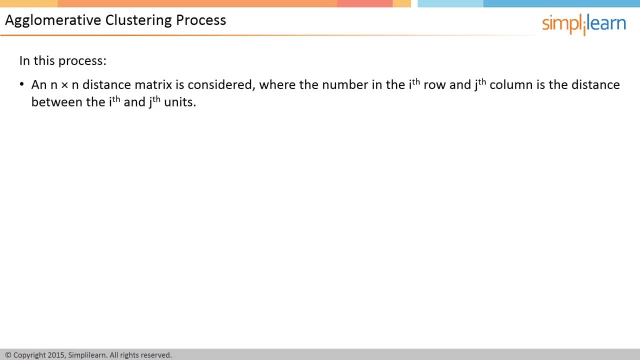 An n times n distance matrix is considered, where the number of the ith row and jth column is the distance between the ith and jth units. The distance matrix is symmetric, with zeros in the diagonal. As the clustering progresses, rows and columns are merged as clusters and the distances between 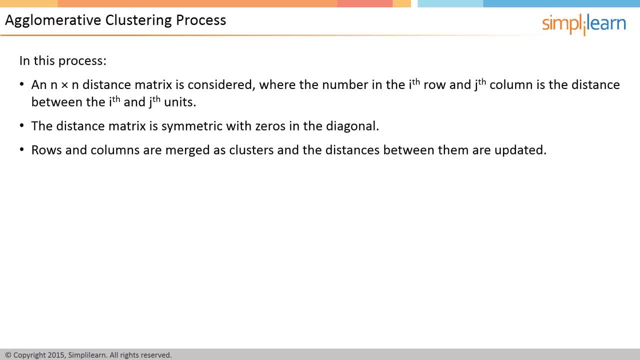 them are updated. You can stop the clustering process based on the distance or number criterion. For agglomerative clustering we use the agns function in the R package cluster. Alternatively, we can use the hclust function in the stats package. 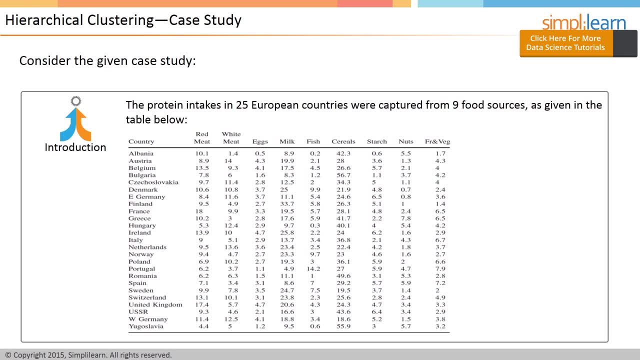 Let's look at the given case study to see how to perform hierarchical clustering. Consider 25 European countries and their protein intake and percentage from nine major food sources. The data is listed on the screen. For example, Austria gets 8.9% of its protein from red meat, 19.9% from milk and so on. 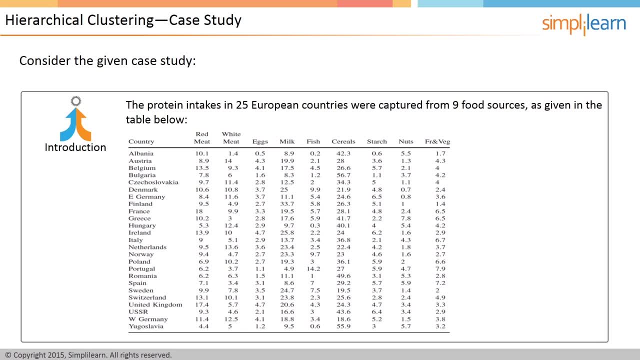 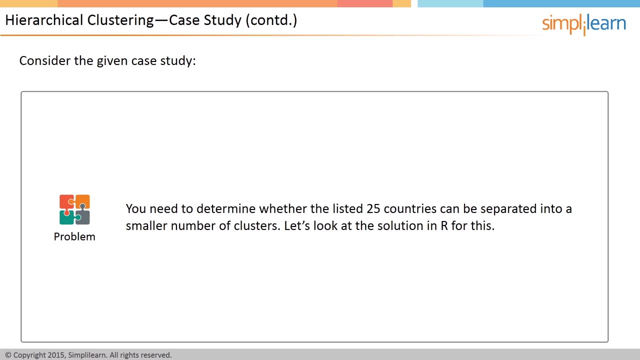 It may well be that Mediterranean countries get their protein intake from certain food categories which are different from the food staples that are favored by North European and German-speaking countries. The result is the same with ourselves for carrot and tackle. Looking at history of data and picture data, you need to determine whether the listed 25 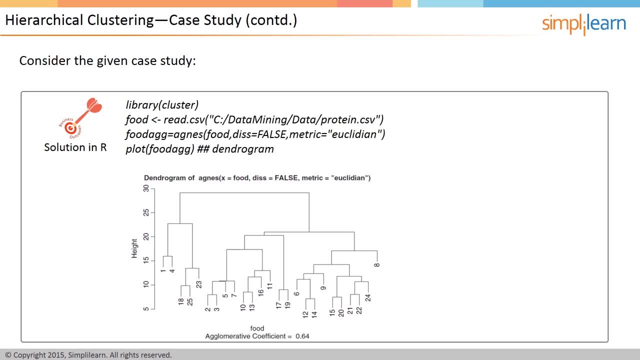 countries can be separated into a smaller number of clusters. To perform hierarchical clustering in R, you need to run the following code: First, load the cluster library into memory by running the command shown on the screen. Read the dataset by using readcsv. 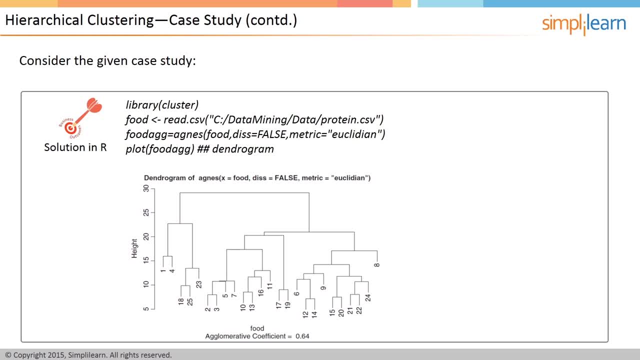 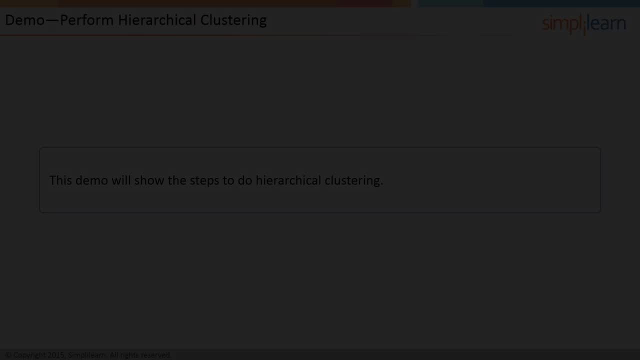 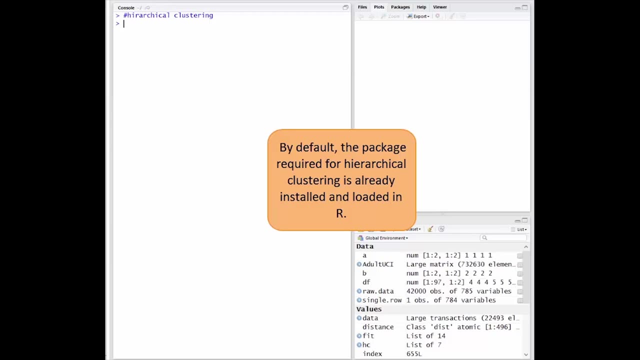 Plot the dendrogram by using the plot function. This demo will show the steps to do hierarchical clustering. In this demo, you'll learn how to do hierarchical clustering. By default, the package required for hierarchical clustering is already installed and loaded in R. 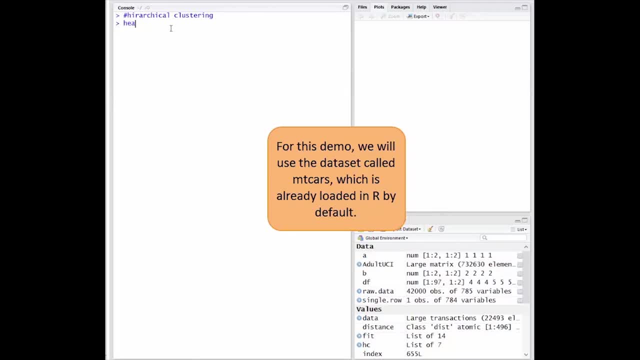 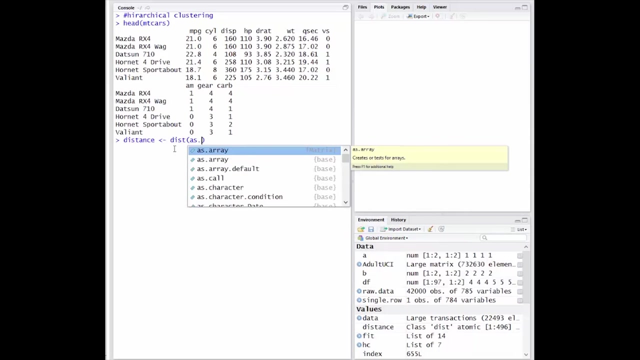 For this demo we'll use the dataset called mtcars, which is already loaded in R by default. Let's compute the distance between rows in the dataset mtcars. We can use the hclust function to do the clustering in that data by distance. 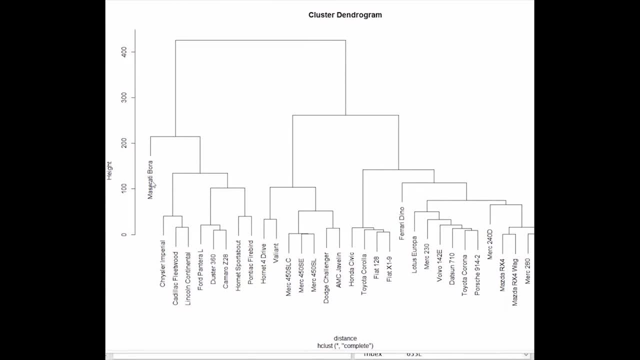 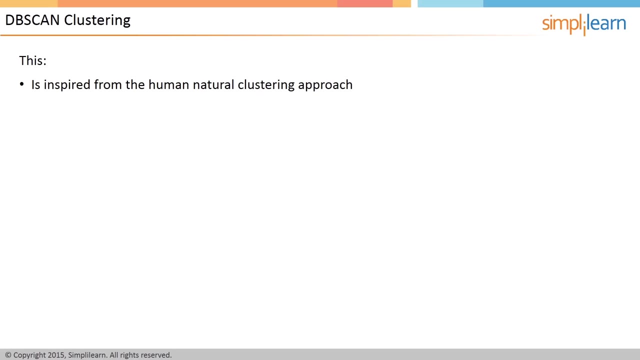 For more options and documentation, we can use the given command. Density-based models of clustering have been vital in identifying nonlinear data based on density. The most popular density-based algorithm is the density-based spatial clustering of applications with noise, or dbscan. Here, clusters are high-density regions that are separated from each other. 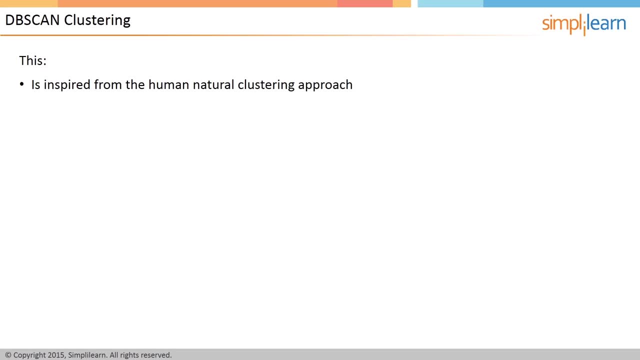 Some regions that have low object density. A cluster is defined as a maximal set of density-connected points. The clusters, and consequently the classes, are easily and readily identifiable because they have an increased density with respect to the points they possess. On the other hand, the single points scattered around the datasets are outliers. 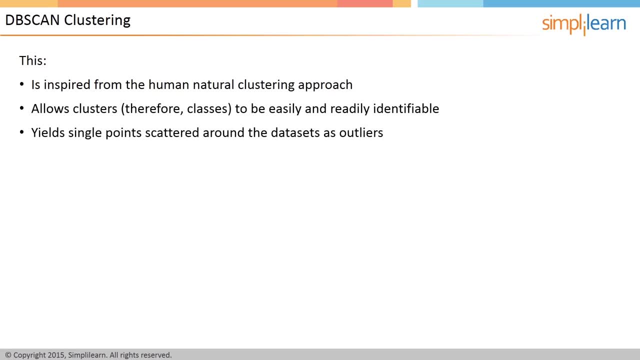 which means they do not belong to any clusters as a result of being in an area with relatively low concentration. The dbscan algorithm requires, at most, to be able to identify the density-based objects in a single cluster. The dbscan algorithm requires, at most, to be able to identify the density-based objects in a single cluster. 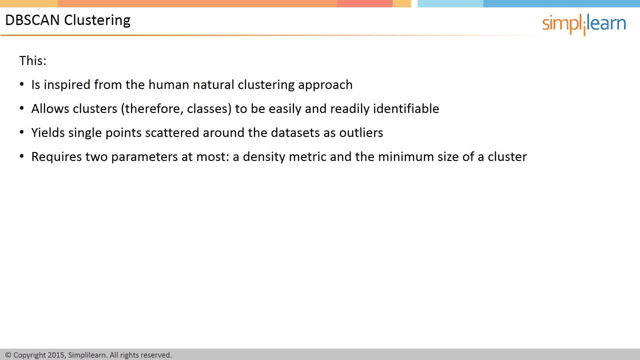 The dbscan algorithm requires, at most, to be able to identify the density-based objects in a single cluster, A density metric and the minimum size of a cluster. As a result, estimating the number of clusters a priori is not needed, as opposed to other techniques, namely k-means. 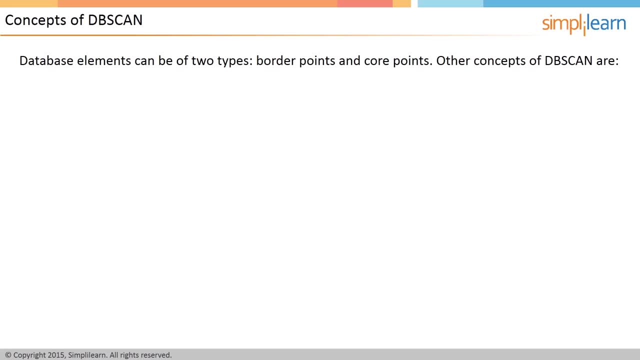 Efficient for large databases. dbscan discovers clusters of arbitrary shapes. Dbscan clusters objects. given input parameters such as epsilon and minimum points, as shown on the screen, This method locates objects within a radius of a certain distance of epsilon from an object. A neighborhood of a point P is a set of all points that have a. 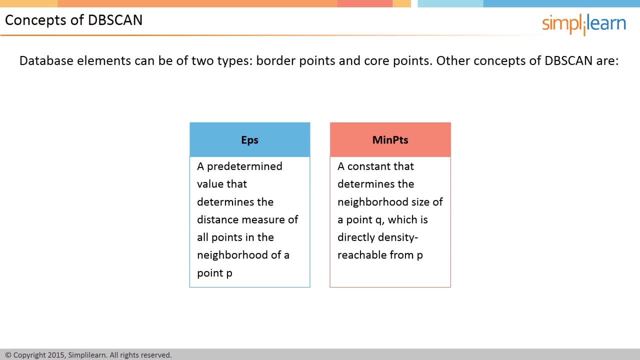 distance measure less than a predetermined value called EPS. Minimum points specify the density threshold of the denser regions. Epsilon neighborhood of an object contains at least minimum points of objects. A point P is directly density reachable from another point Q if it belongs to the neighborhood of Q and Q's neighborhood size is greater than a given. 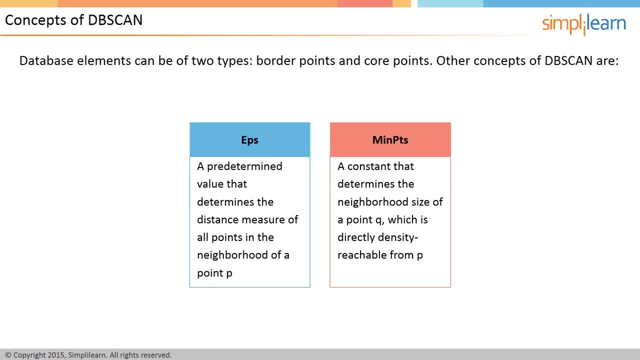 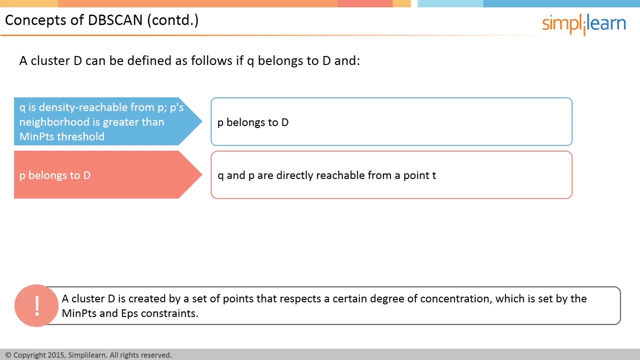 constant minimum points. To determine these constraints, compute the distance from a point to its kth nearest neighbor and plot the sorted values. A cluster D is created by a set of points that respects a certain degree of concentration, which is set by the minimum points and EPS. 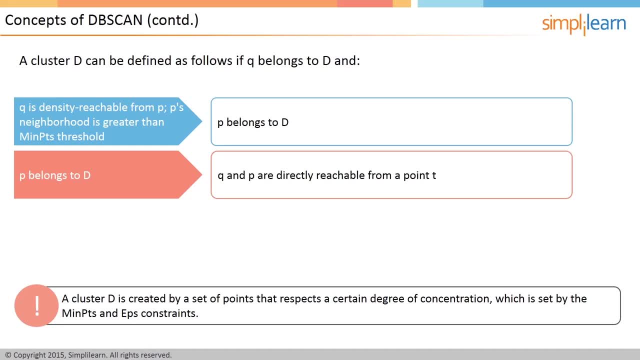 constraints. DBScan uses the concepts of density, connectivity and density reachability. A point P is said to be density reachable from a point Q if point P is a density reachable point. A point P is said to be density reachable from a point Q if point P is within epsilon distance from point Q and point Q has sufficient number of points in its 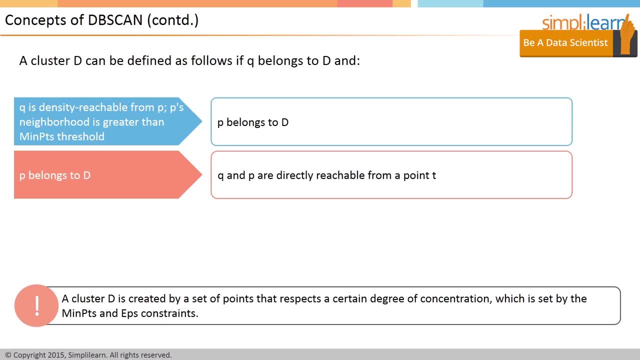 neighbors which are within distance. epsilon Points P and Q are said to be density connected if there exists a point R which has a sufficient number of points as its neighbors and both the points P and Q are within the epsilon distance. If Q belongs to D and if Q is density reachable, 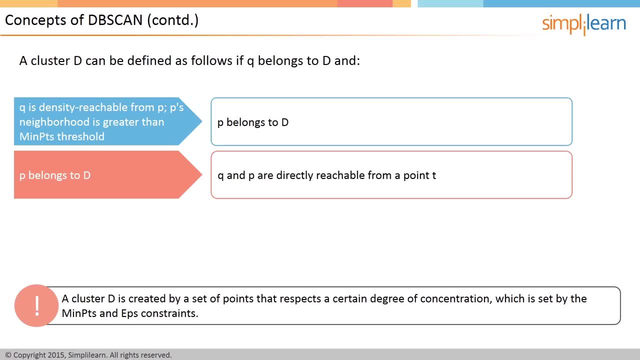 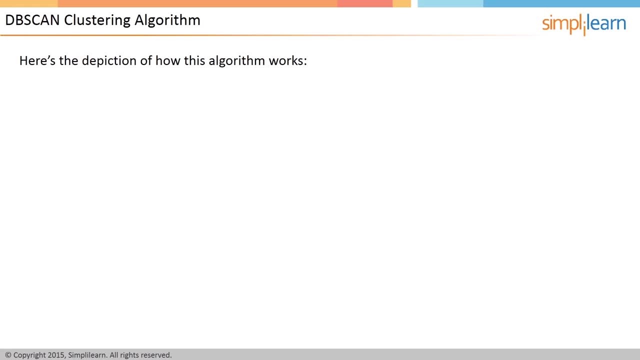 from P and P's neighborhood is greater than the minimum points threshold, then P belongs to D. Given the constraints, the objects can be classified into core, border and noise points. Core points lie in the cluster's interior. A point is defined as a core point if it has more. 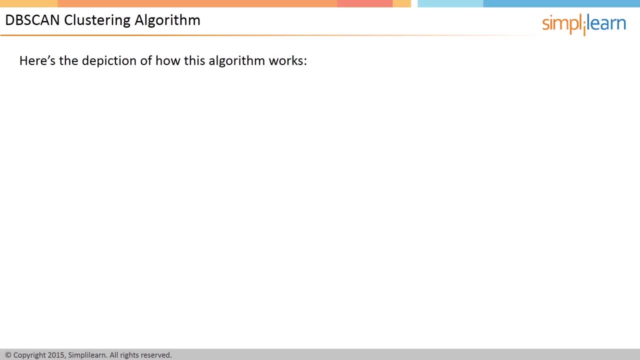 than a specified number of points or minimum points within EPS. A point is defined as a border point when it has fewer than minimum points within EPS but is in the neighborhood of a core point. A point is defined as a noise point if it is neither a core point nor a border point. The algorithm of DBSCAN is as follows: Select an. 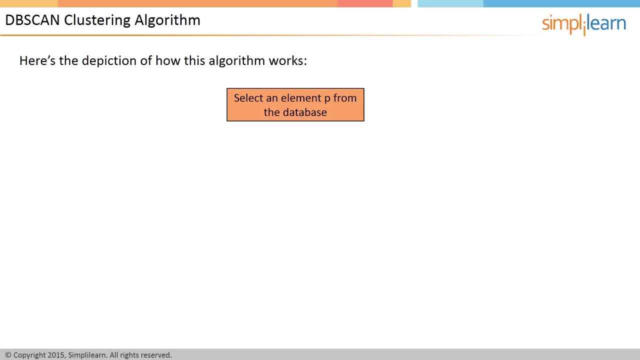 element P from the database. You need to retrieve all points density reachable from P with respect to epsilon and minimum points. If P is not a core point, mark P as noise. If P is a core point, mark P in the cluster and call the expand cluster function. The expand cluster is a recursive.